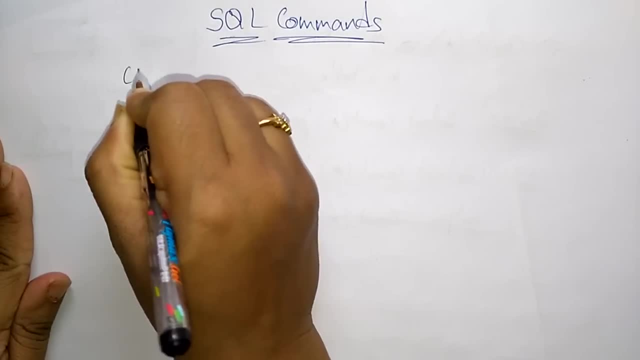 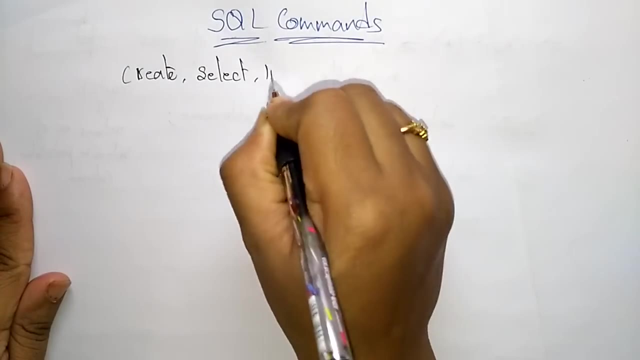 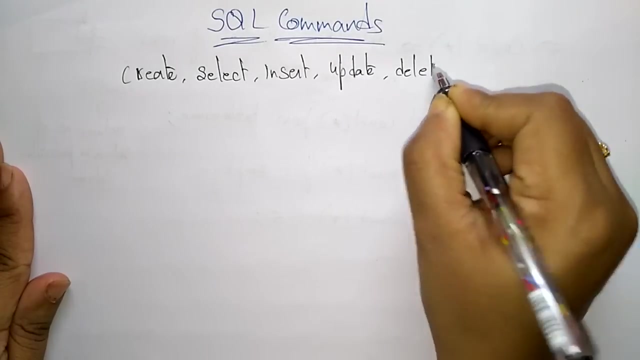 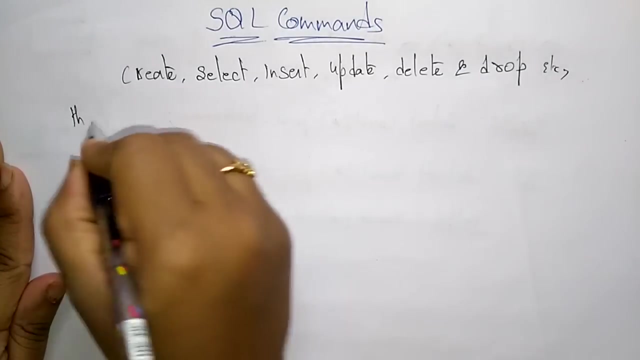 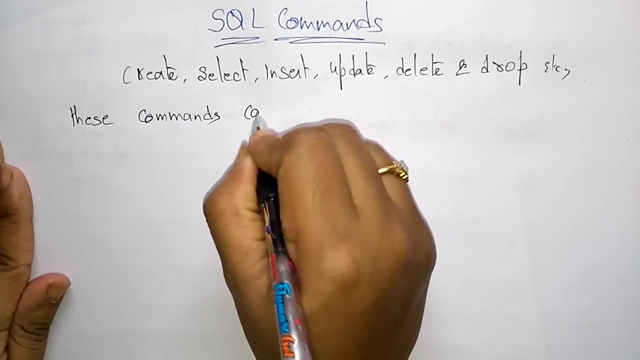 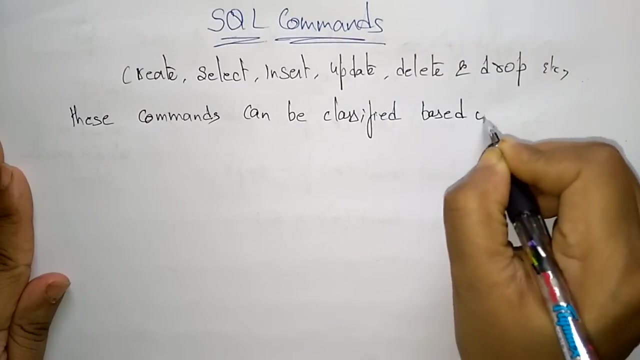 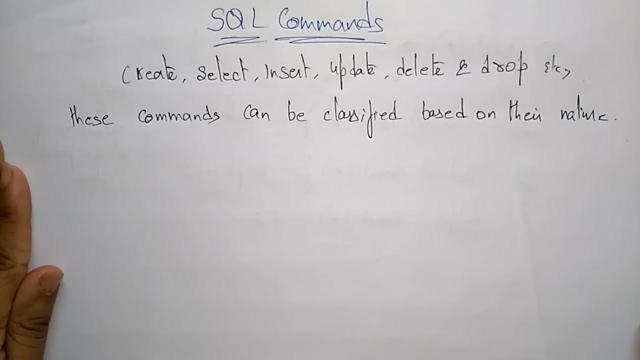 Actually, some of the commands like create, select, insert, update, delete and drop, So these commands, etc. These commands can be classified. can be classified based on their nature. based on their nature means in what type of language we are using. So, based on their nature, we can create the table. 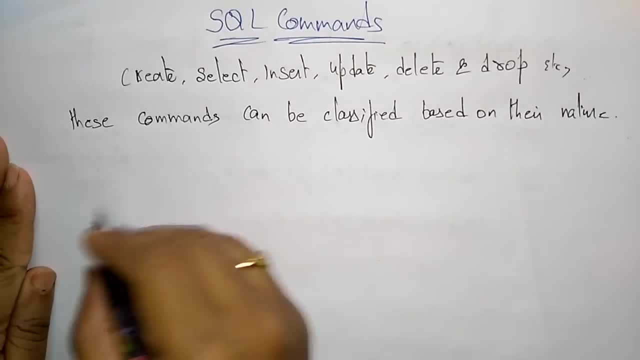 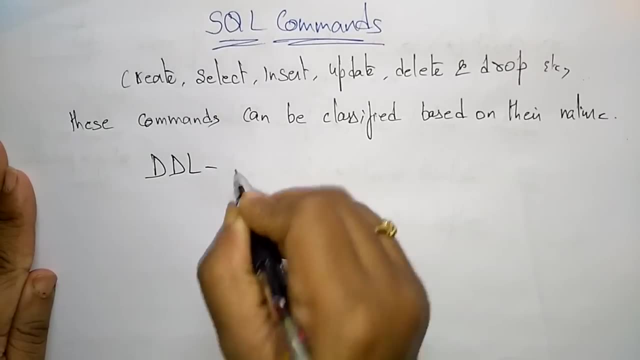 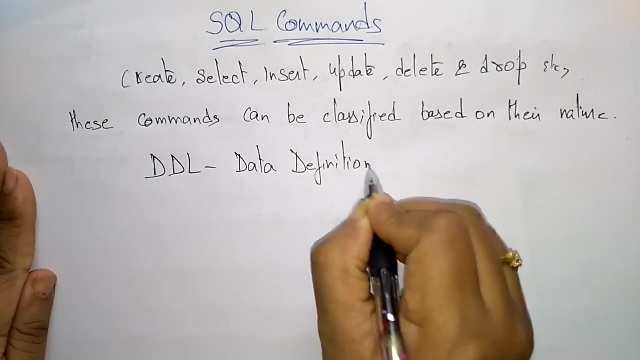 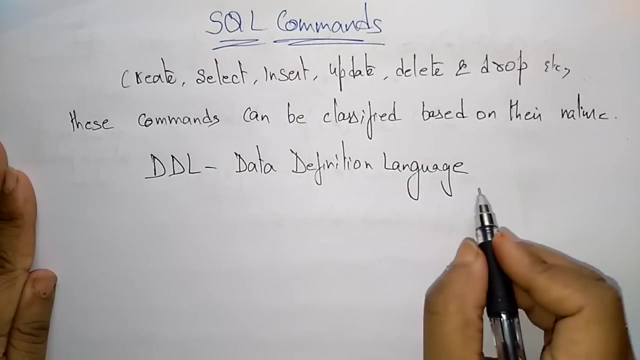 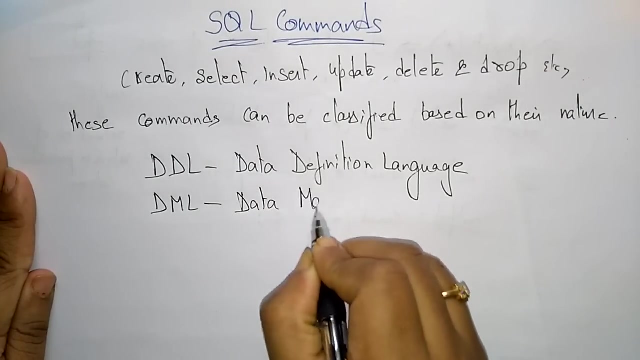 means based completely on the user requirement. So different languages that are used in the SQL commands or the DDL means: DDL: D for data, D for definition, L for language. DDL commands means data definition language. Next, DML commands: data manipulation: M for manipulation. 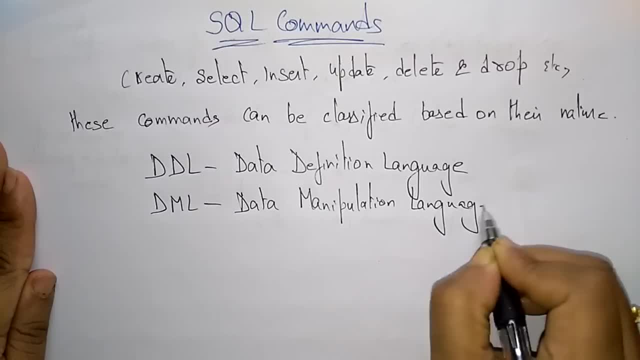 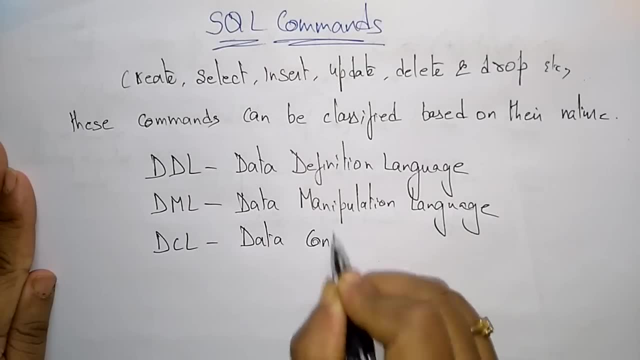 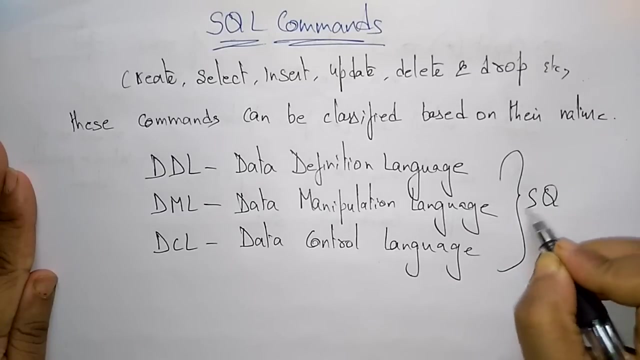 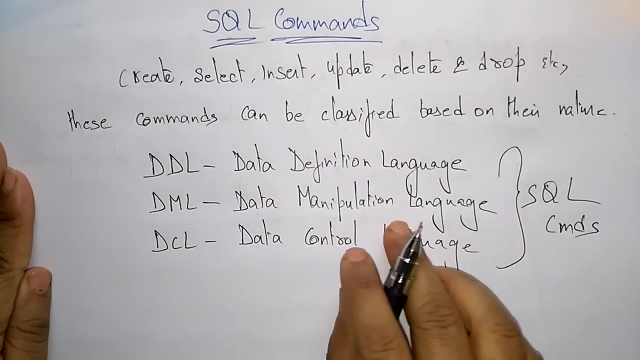 L for language and the next DCL, L for data control, C for control and L for language. So complete structured query language commands divided into these three types. So data definition language, data manipulation language and data control language. Let us see one by one. 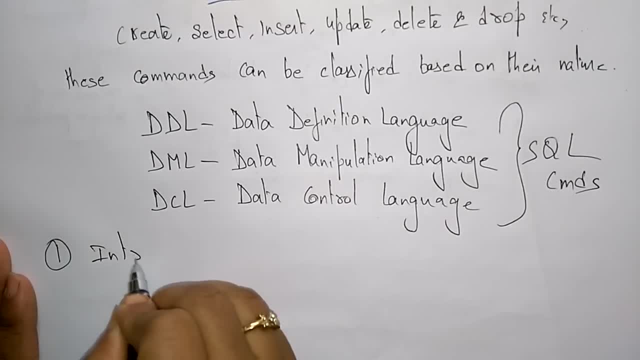 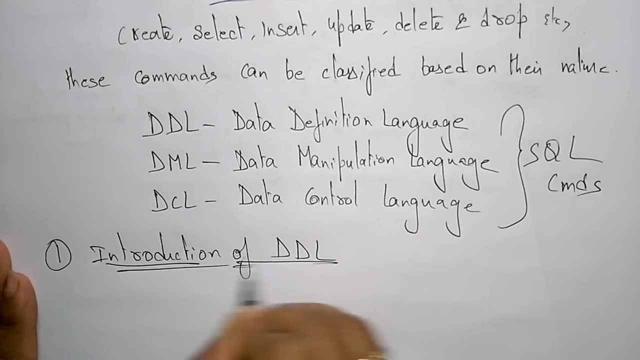 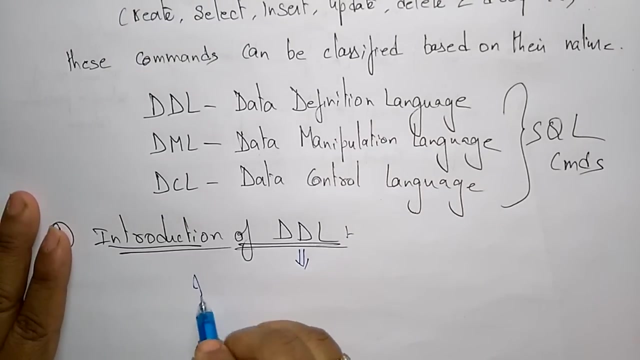 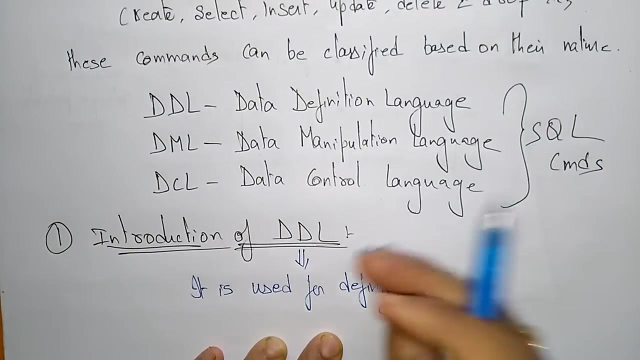 So the first will take the introduction of the data data definition language. so what is the main use of this data definition language? so this data definition language, it is used for defining, so the name is self is saying data definition, so a definition will be present in that. so it is used for defining. 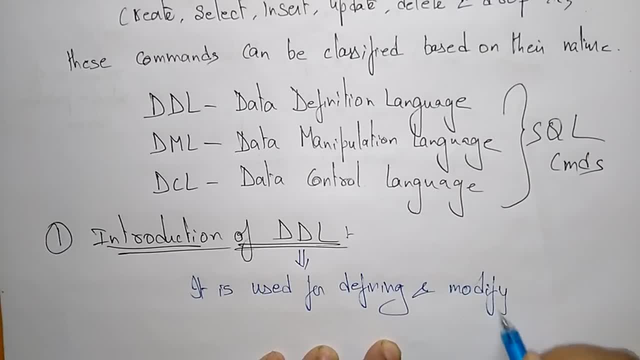 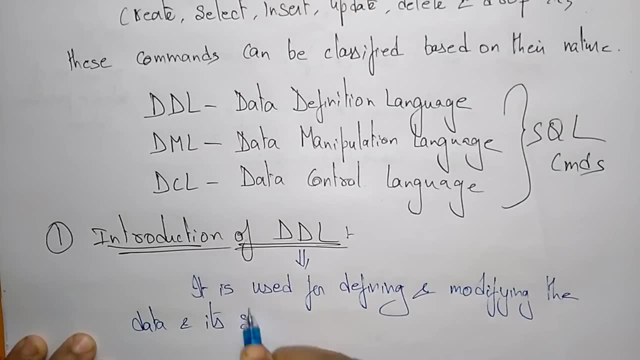 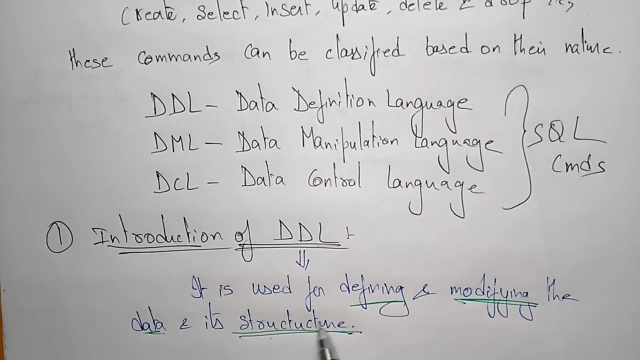 and modifying the data, data and its structure. so the main use of the commands that are used in the data definition language, or use it, to defining and modifying the data, as well as its structure- okay, structure- and also it is used to build. let me write: it is also used to 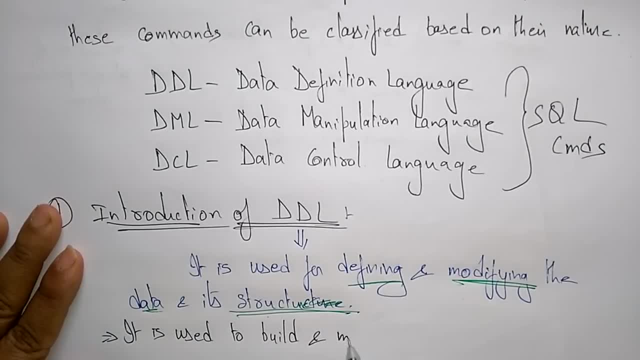 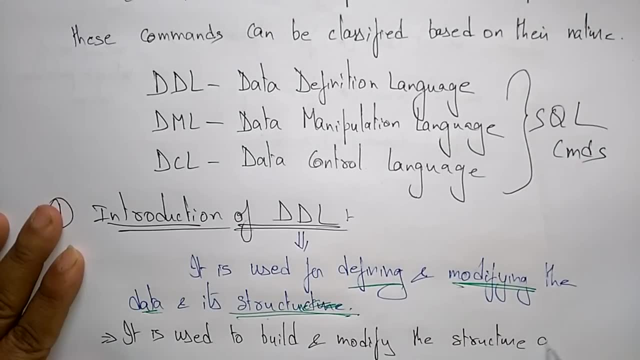 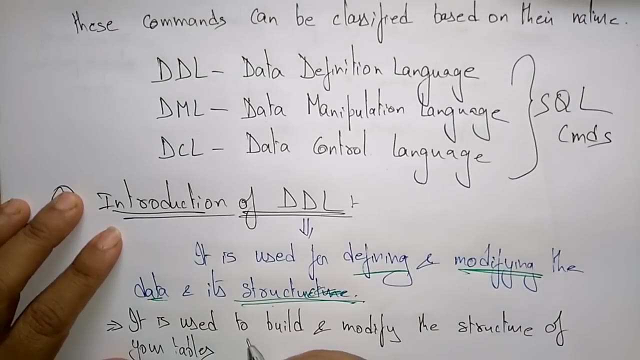 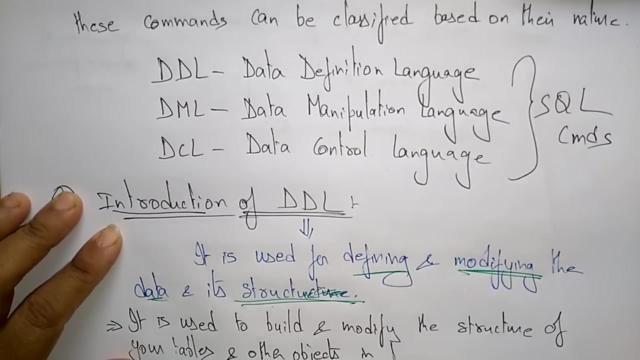 build and modify the structure, modify the structure of your tables, whatever the tables you are creating, so that will be modified. and also other objects will be modified, other objects in database. so then, the main use of the data definition language is the, whatever the commands, that are, the sql commands, are used in. 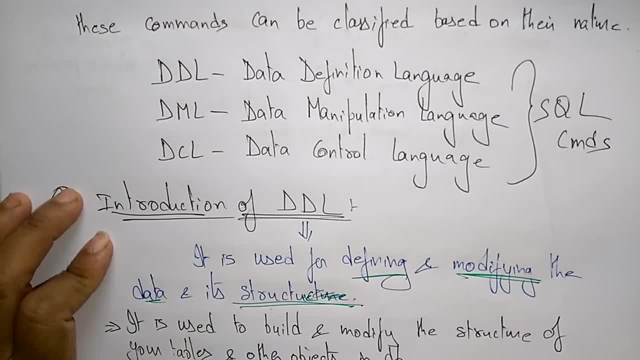 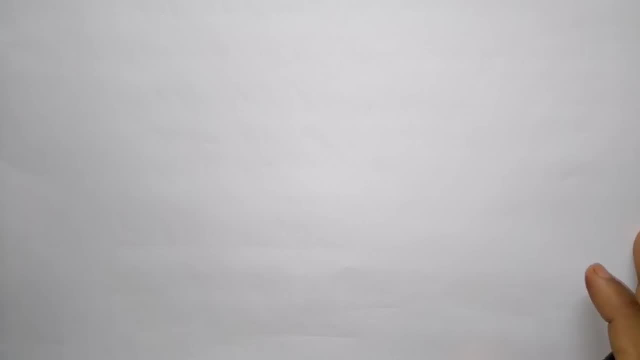 the data definition language or use it to defining and modifying the data, as well as the complete structure of the commands. so let us see what are the commands that are used in the data definition language. commands used in the data definition language. so those are. first, one create. 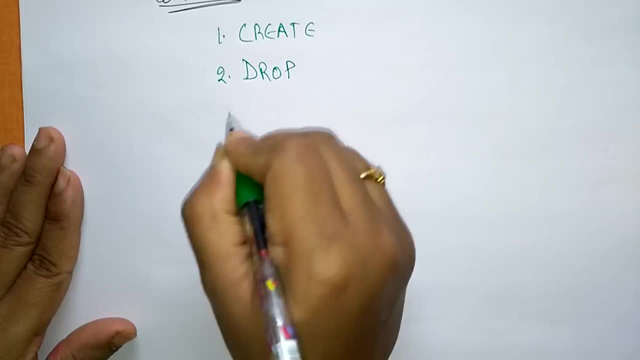 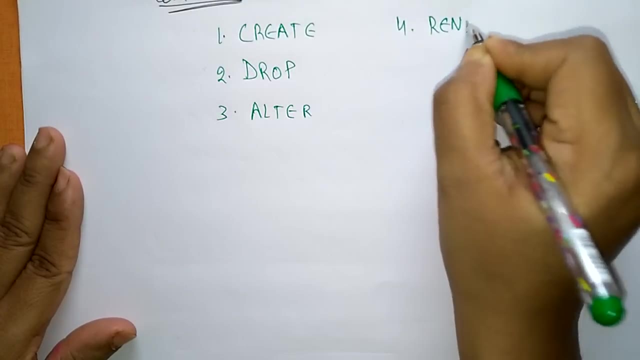 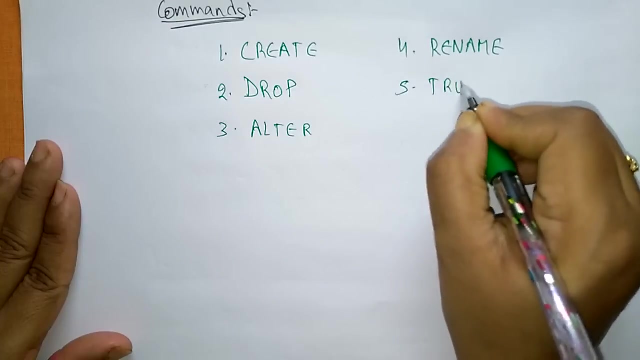 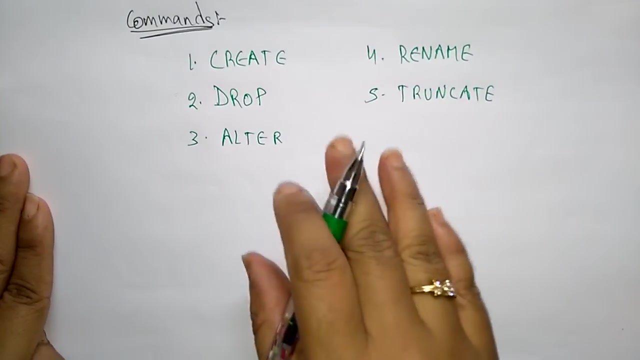 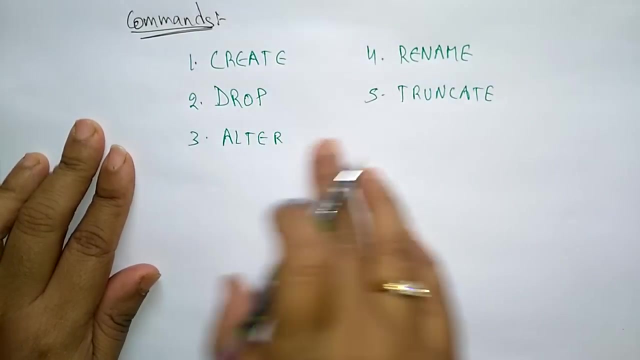 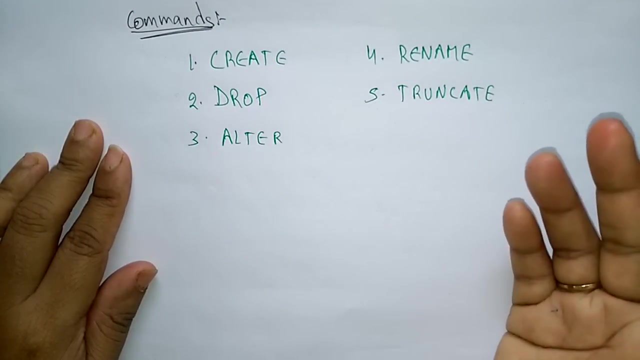 second, drop, third, alter, fourth, rename, fifth, truncate. so these are all these five commands. you call it as a data definition language. why we call only these five commands as data definition? because this create, drop, alter, rename, truncate- these commands are used for defining. so create is used to defining the table and modifying the data and its structure. so 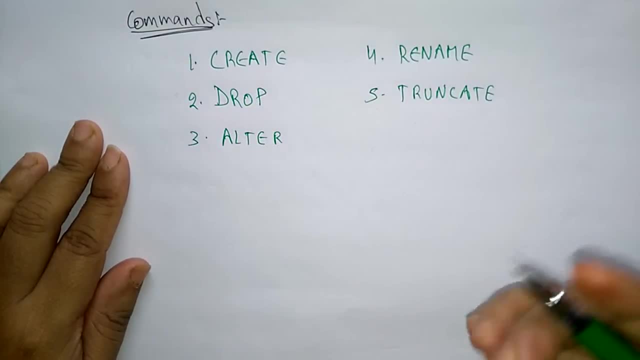 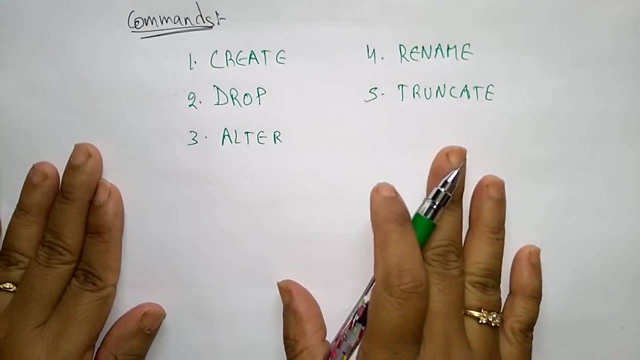 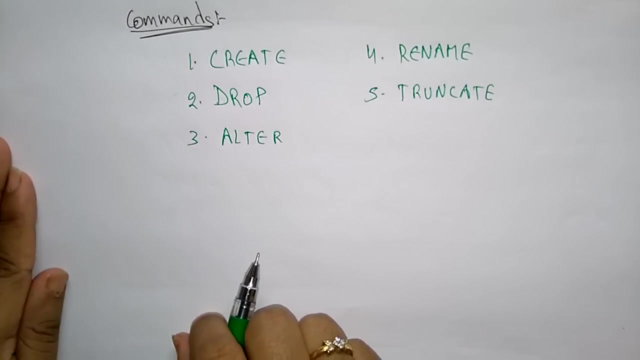 modifying and define, uh, modifying the data and structures will be done by the drop, alter, rename truncate. so this is the these the commands use it to modify and defining the data and its structures in the table. so these commands you call it as a data definition, language commands, so data definition. 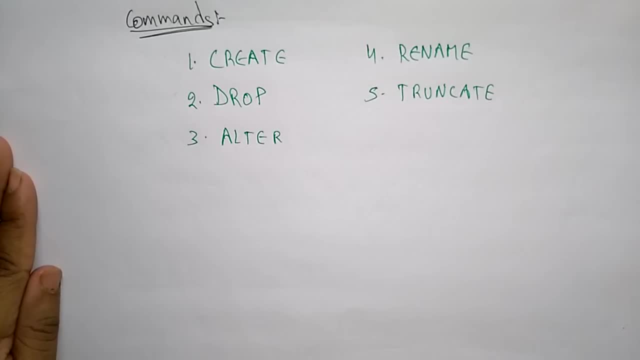 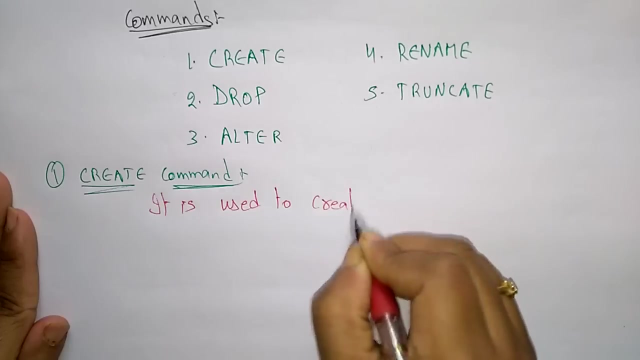 language has predefined syntax for describing the data, so let us discuss one, one by one: command and create command. so what is the use of the create command? what is the syntax for this? let us see: it is used to creating objects in the database, so it creates the objects in the database. means: 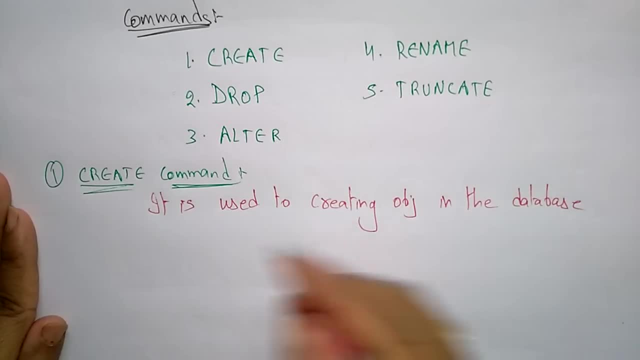 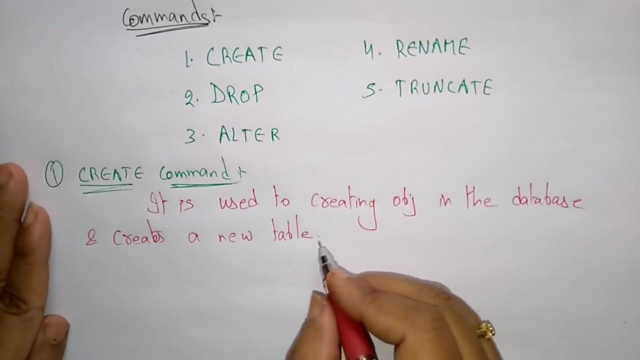 it is creating the fields in the database, records in the database and also it creates a new table. so in the existing table it is used to add the objects and at the same time it also creates a new table in the database. so let's write the syntax for this: create command. 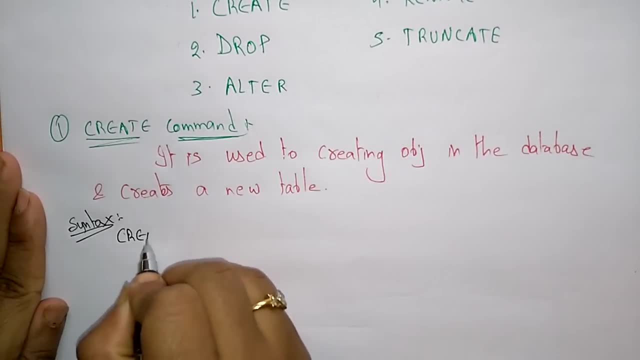 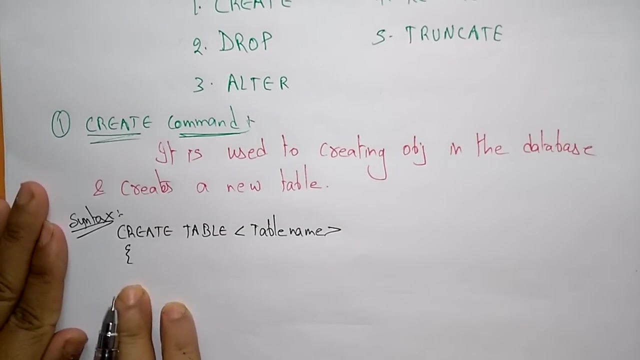 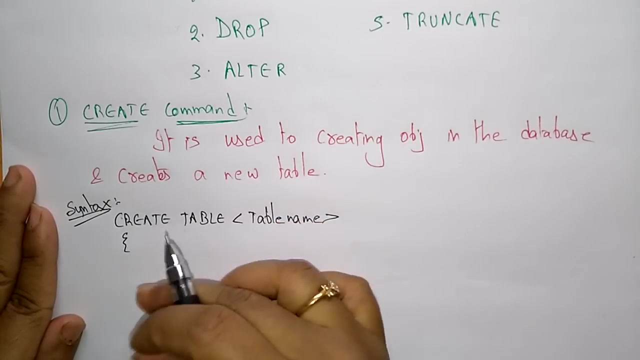 so what is the syntax for this? create table. so here you have to write the table name, the relation name, whatever you want. you write the table name and let's abrases, curly braces. so for creating, you have to write everything. the definition means this is a data definition and everything the definition within the braces, just like a function. 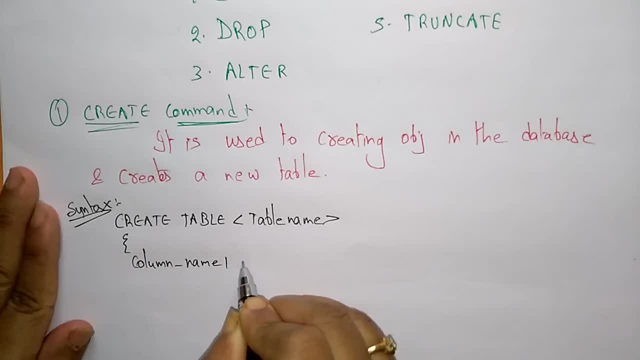 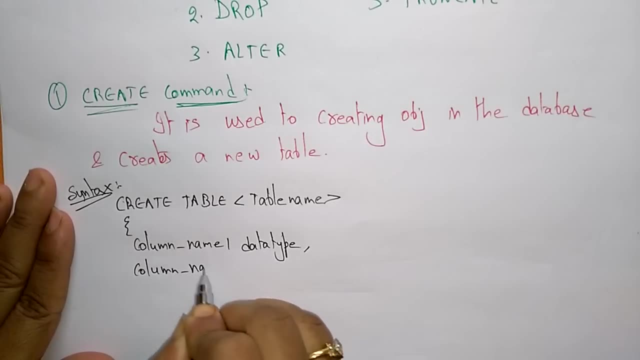 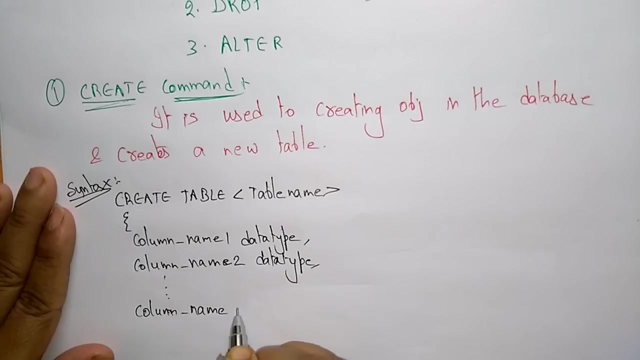 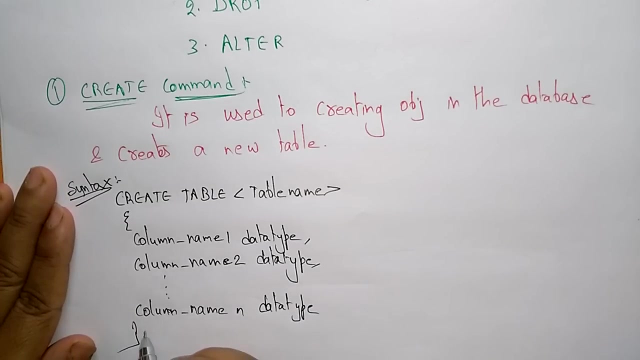 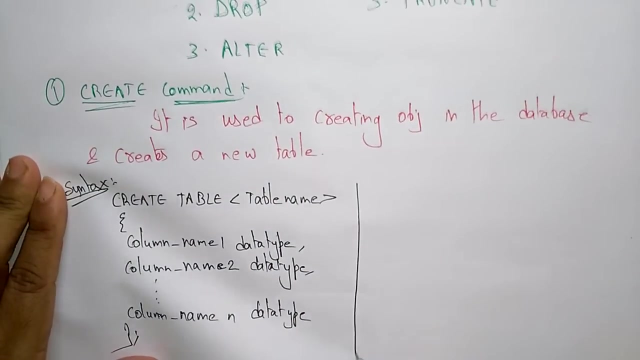 column name. one data type comma. column name: one data type comma. column name: one data type comma to data type. up to column name and data type. close the braces semicolon just like a class. so this is a create command, the syntax for the create command. now let us see the example for this. 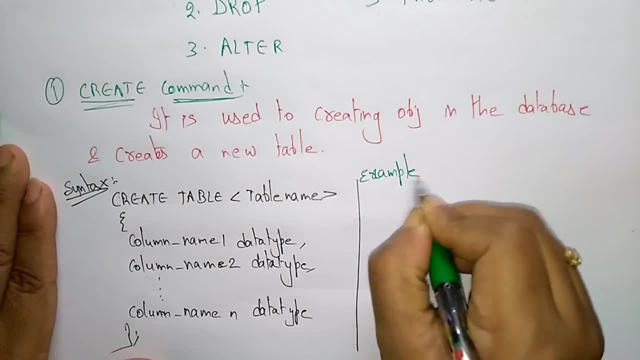 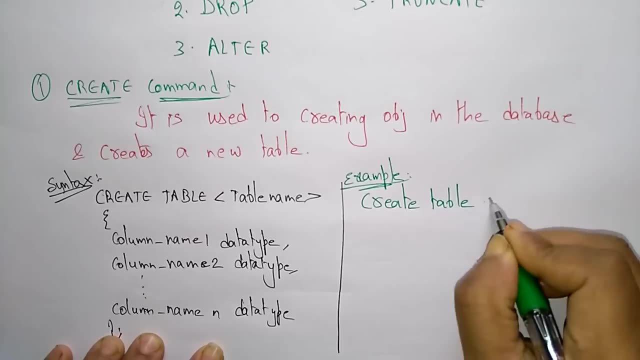 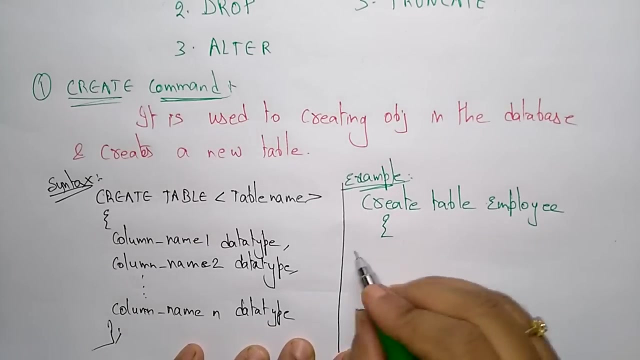 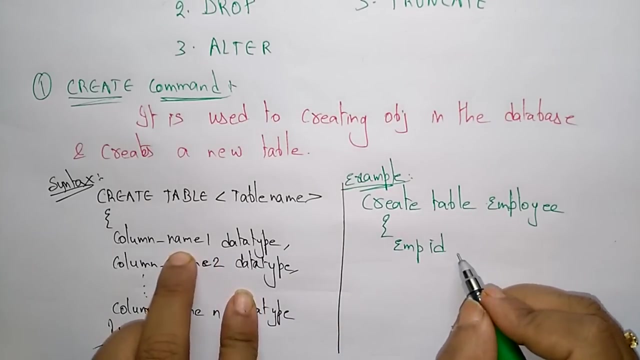 so create, so table the table name. here I am writing employee. employee is a table I'm creating the fields in the table means attributes, employee ID and the data type. a column name one- that is the first field- is employee ID and the data type. here I am. 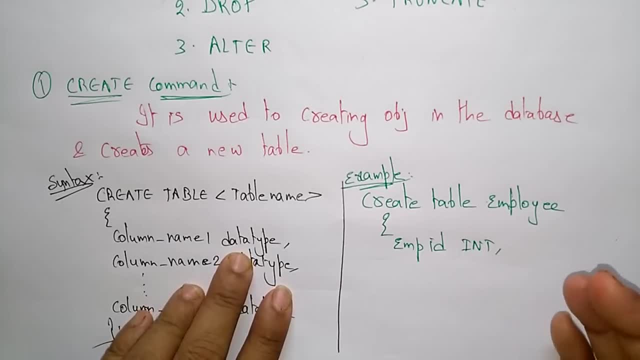 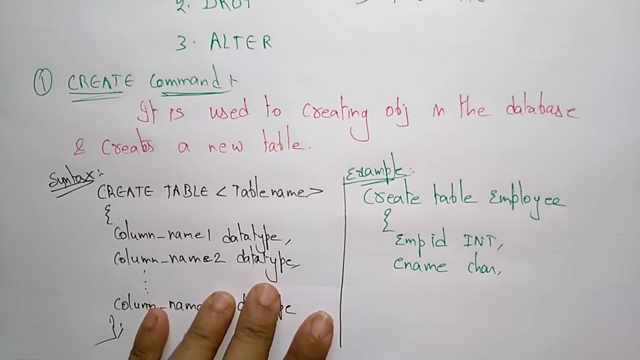 using int, because only the integer values you can enter for the employee ID, like one, two, three zero zero. one, one zero zero, two, like that. only the values that should be integers. ename: employee name should be a character, so always the name should be a character. age: age is int integer. 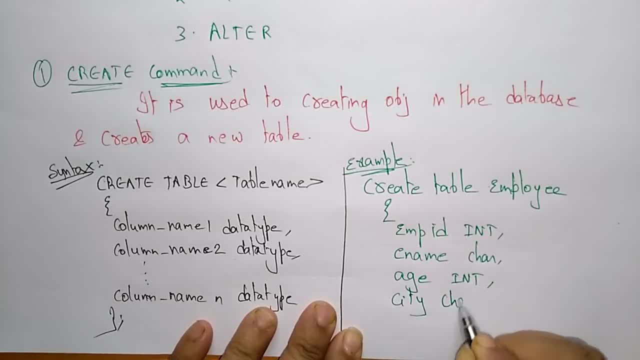 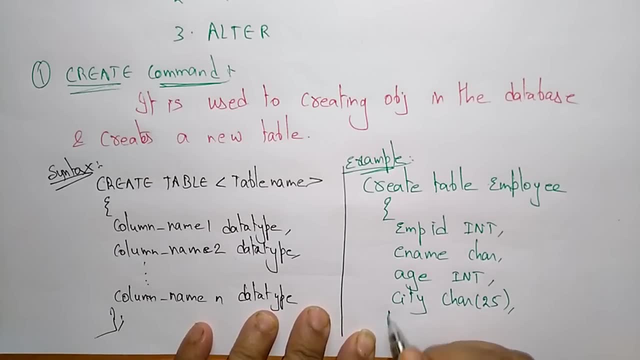 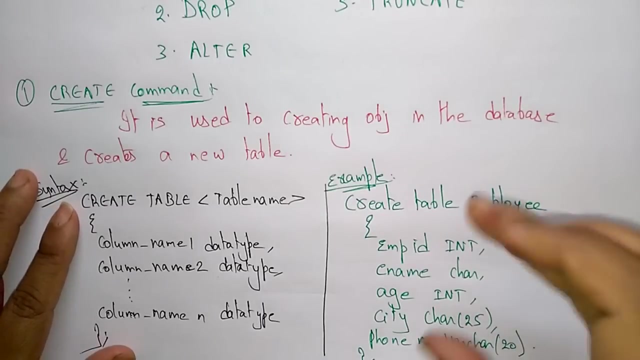 and this coming to city, city character. I'm mentioning the size of means: up to 25 characters. you can enter the name of a city and, coming to the phone number, phone number should be varchar and close the creative. so this is how to create a table. so whenever I enter this structured command, 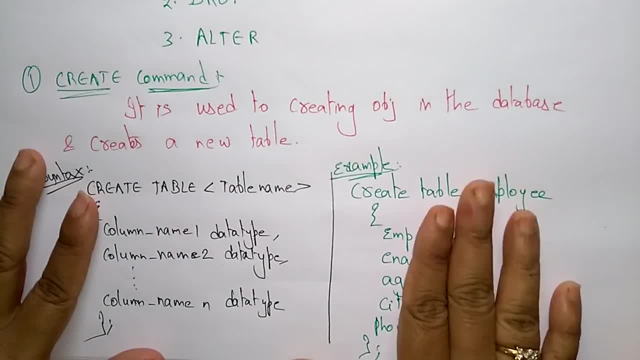 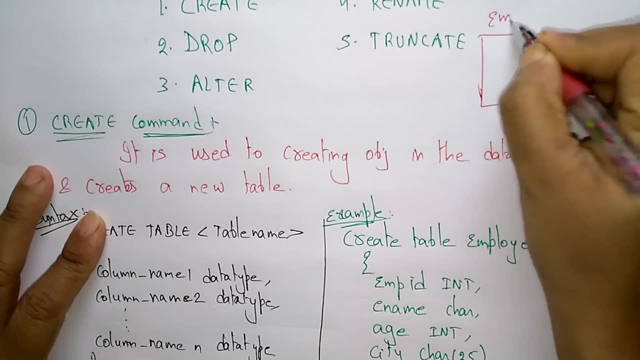 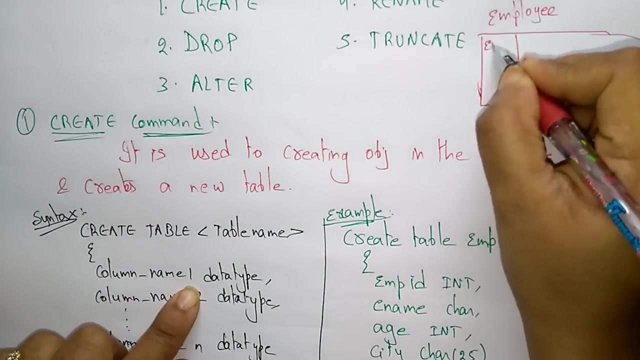 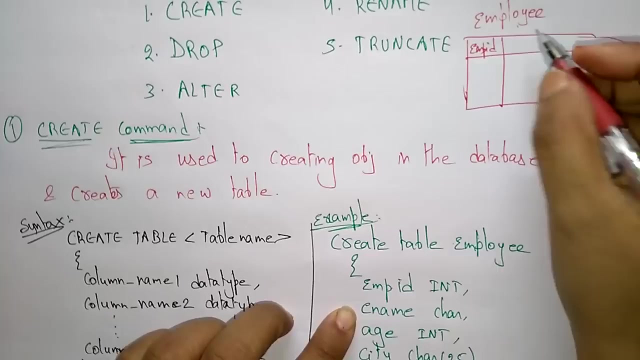 means and whenever I entered this command, whenever I create this command, the table that I that it is created is the table name, is the employees, the table name, so the fields. the first column name is the employee ID- a structure is created in the database- but the table name employee. the second is: 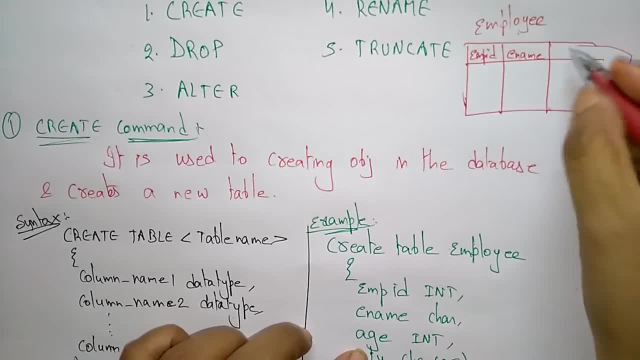 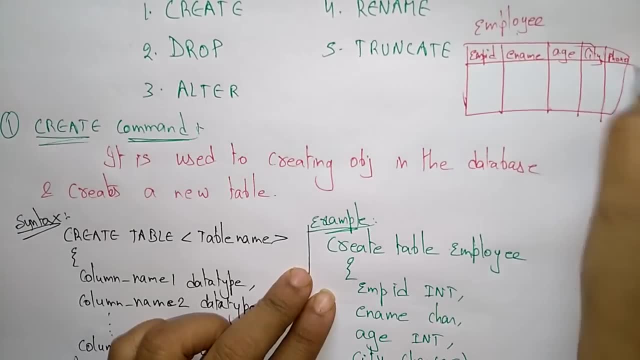 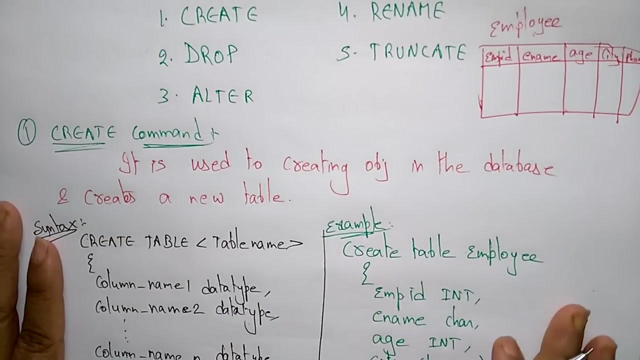 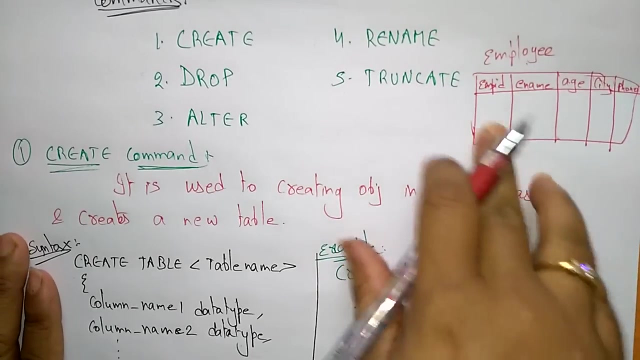 second field is ename. third field is age, city and the phone number. so these are the fields. only the table was created, not the values. that i values are not inserted in the tables. only here i created a table with these fields total five fields. so this is a structure that is present in the database. 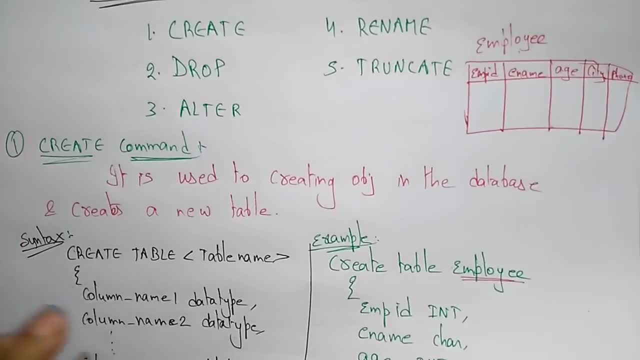 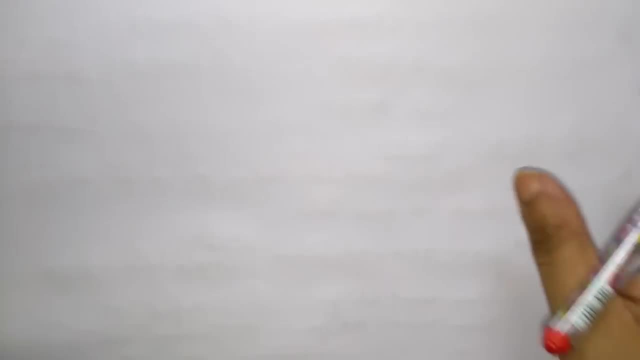 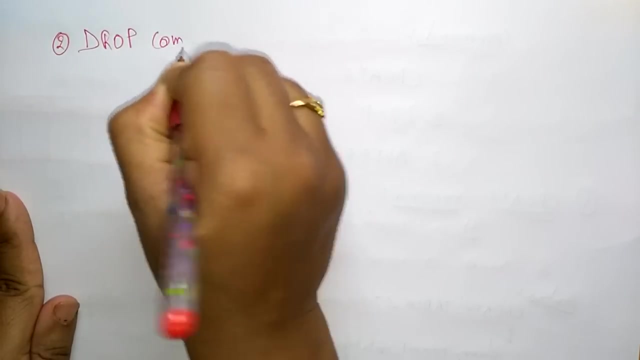 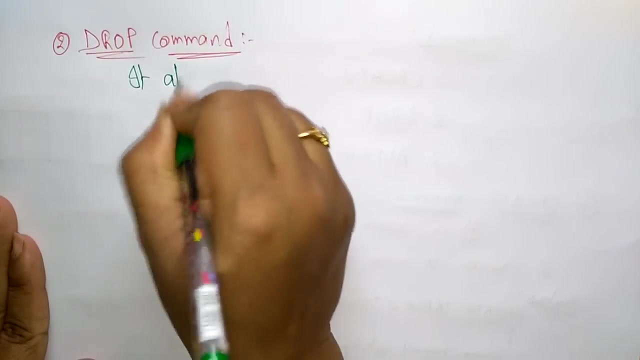 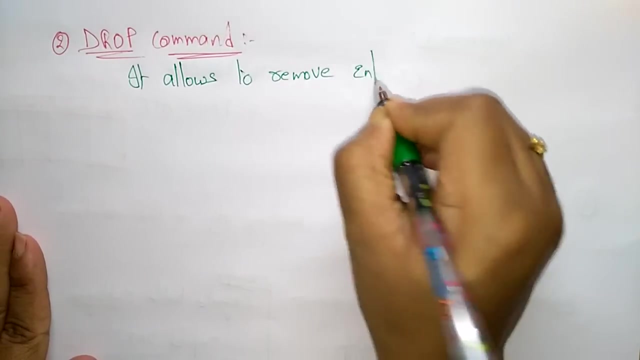 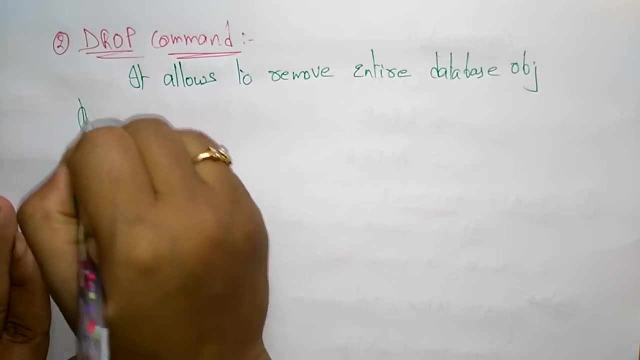 so whenever i written this command. so this is about the create command. next coming to the drop. so what is the syntax for the drop command? so drop is one of the data definition language drop command. it allows to remove entire database objects from the database. so it removes the entire database objects, whatever the objects. 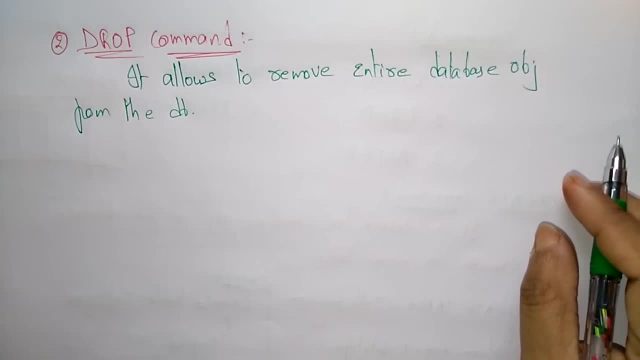 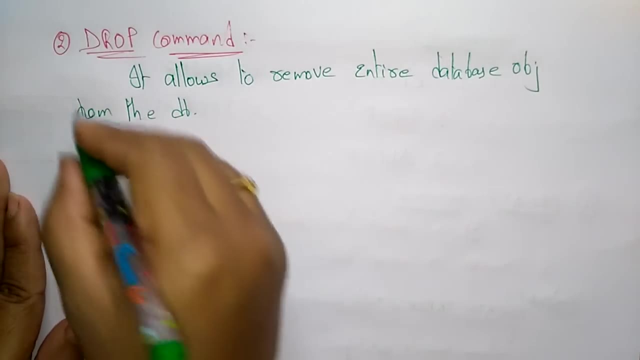 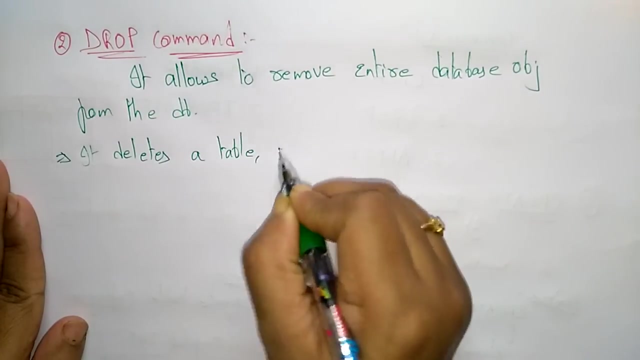 we created. what are the fields that i created there that will be removed. so the table will be exist, but the fields will be removed. so it removes the entire database objects from the database and it also delete. it deletes a table, oh sorry. it also deletes the table index or view also completely. 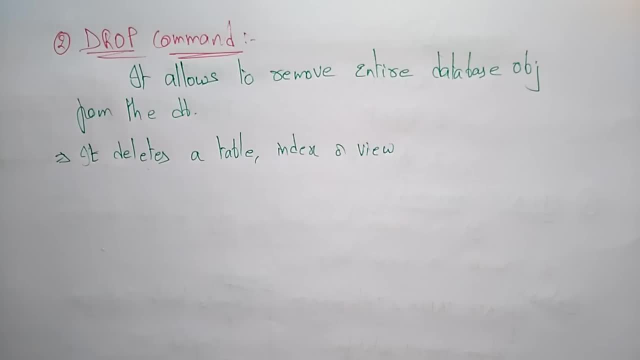 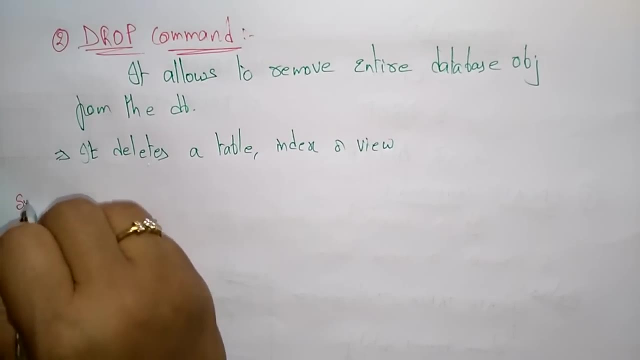 whenever i use the drop, it completely deletes the table and the fields, whatever it present, and the index or we. everything will be deleted. now let us see the syntax for this. just you have to write drop table table name. so whenever you write this, the table complete, the table will be dropped. or you can drop the database, also drop. 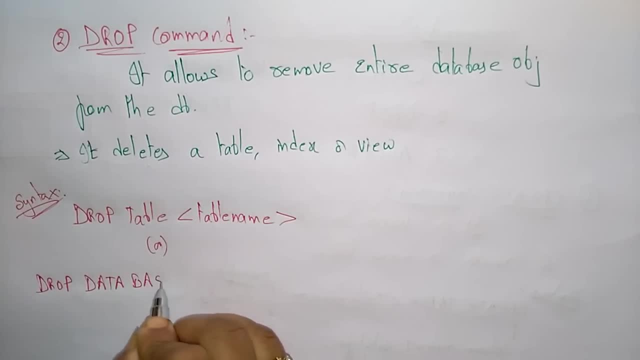 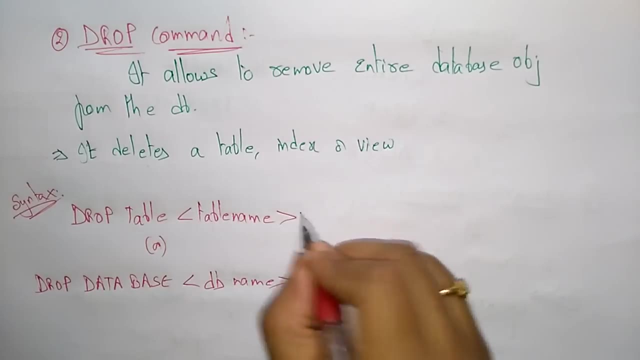 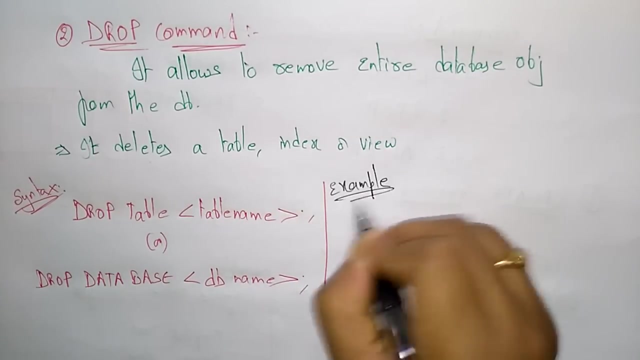 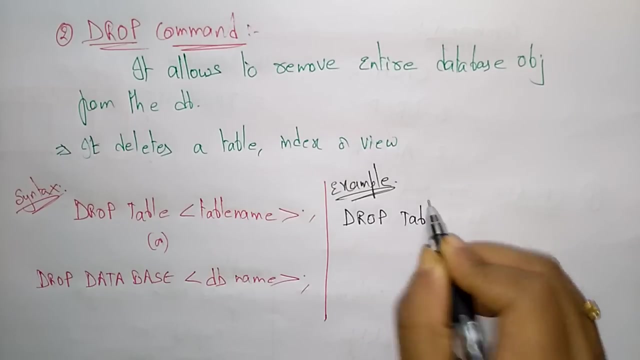 in the other case usable- and then referral. I think i take a character in the length field right now because takeaway it if you don't want. so below in visiting the fool slot, it works. so you have to do what this means. drop table: if you want, you can just create the book title as it is, like what you definitely. this is because 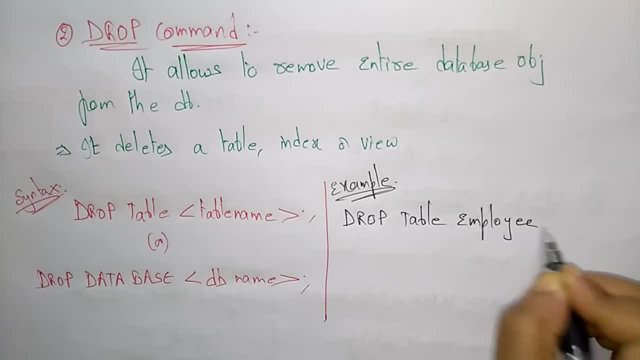 here, use the mark up info, google see all action photo, or here you know, can change un э d e d l, two key facilitators. so here, like i just say, actually open your detectiveек then. then it will be different with random thing data base, that is a database name you have to write. so this will be the syntax and coming the example. irrelevant, j incapable. so whatever, i created the employee table previously. drop table employee. so before dropping you have to create the table otherwise. so before dropping you have to create the table and you have to adapt the data. that is one Serbia, for example. here it gives youelia set两utentingo correct first. 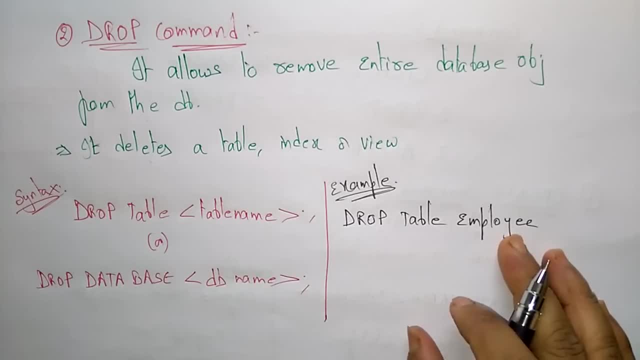 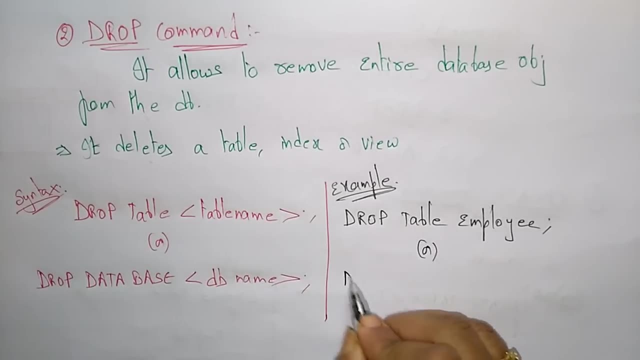 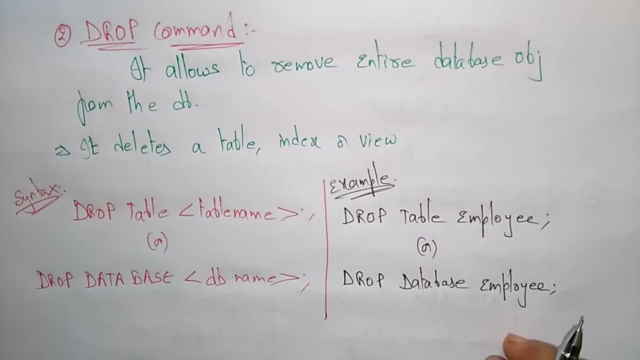 if the table is not there, you are not. this syntax will be getting error. so drop table employee, so the table will be dropped. or else drop database employee, so complete database will be dropped, or else a particular table in that database employee will be dropped. okay, the table name. 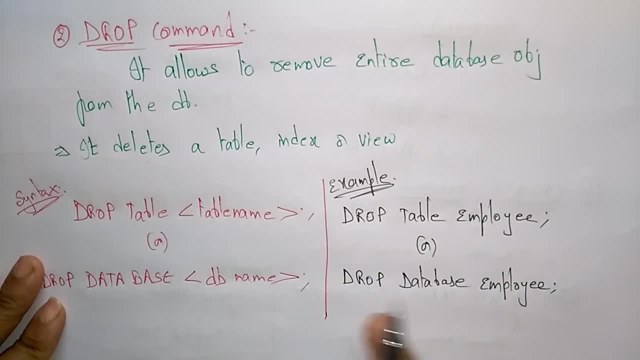 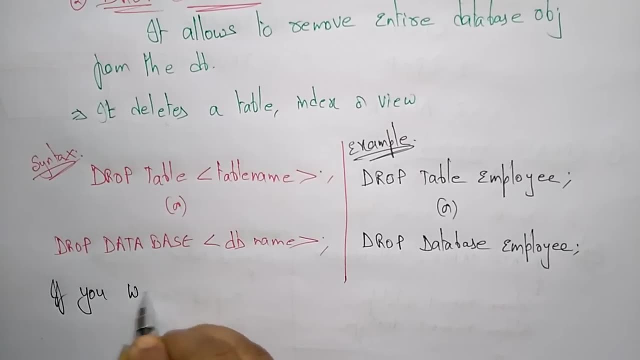 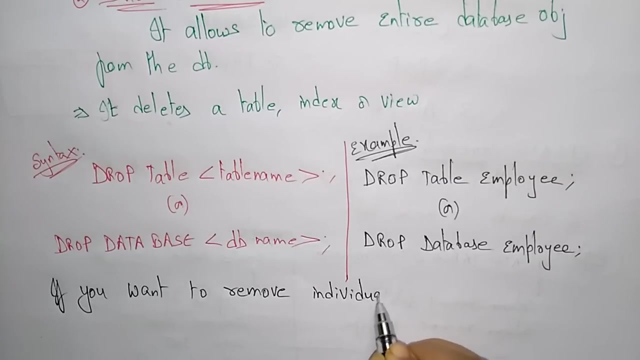 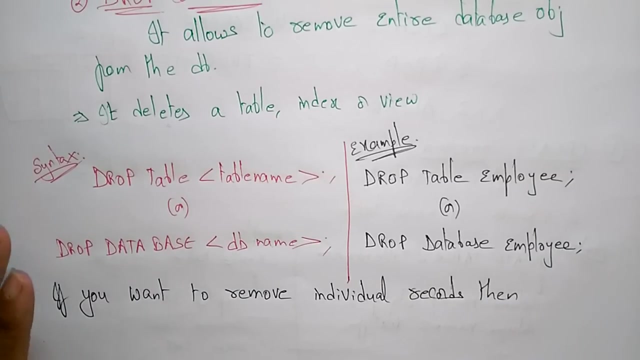 and the database name may be same, so drop table table name or drop database employee. so if you want to remove, if you want to remove individual records, then if you want to remove an individual record in each table, then you can use delete command, not for complete table dropping, if you want to delete only particular.